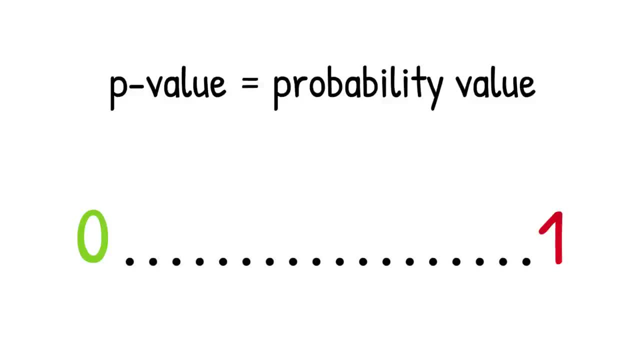 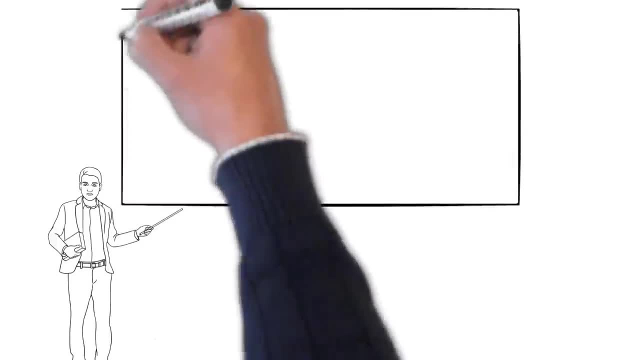 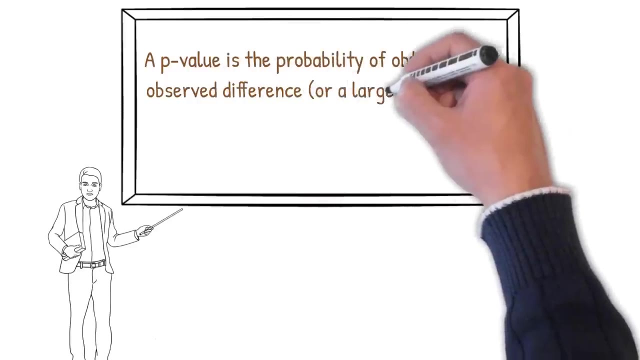 any value between 0 and 1.. But what exactly does this number represent? The official definition of a p-value is quite difficult to understand. A p-value is the probability of obtaining the observed difference, or a larger one in the outcome measure, given that no difference exists between treatments in the population. 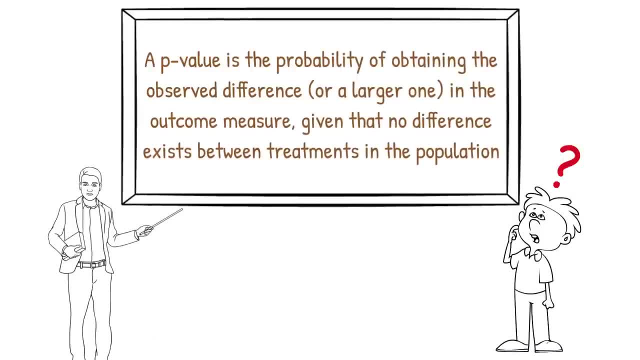 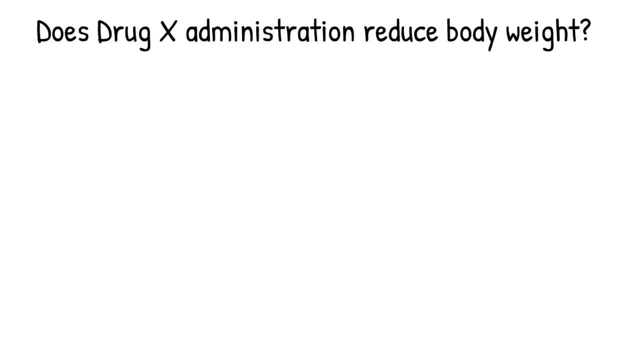 So the best way to explain what a p-value is is to use an example. Let's say you want to perform an experiment to see if a new type of weight loss drug, drug X, causes people to lose weight. So you randomly sample a collection of volunteers and randomly assign them. 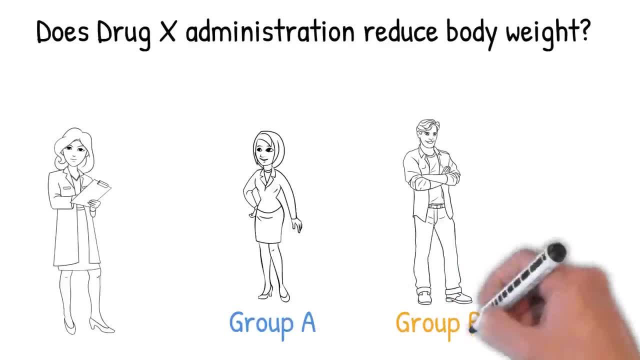 into two groups: group A and group B. By the way, if you don't know the difference between a sample and a population, it might be worth checking out the previous video. Group A is a placebo, In other words, this contains no active ingredients. 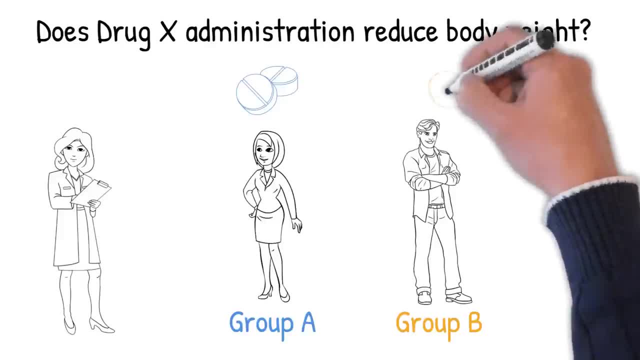 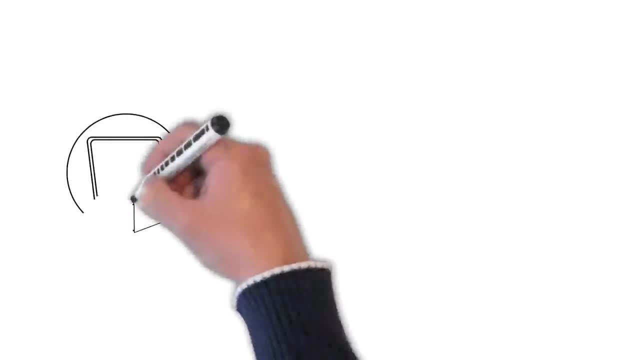 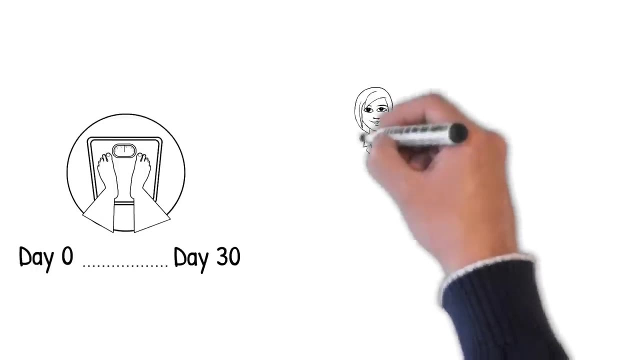 Group A are therefore the control group And you give group B the new drug, drug X. The participants are weighed at the start of the study and at the end of the study And this way you can work out the body weight difference. At the end of the study you work out that group A's average body weight difference was zero. 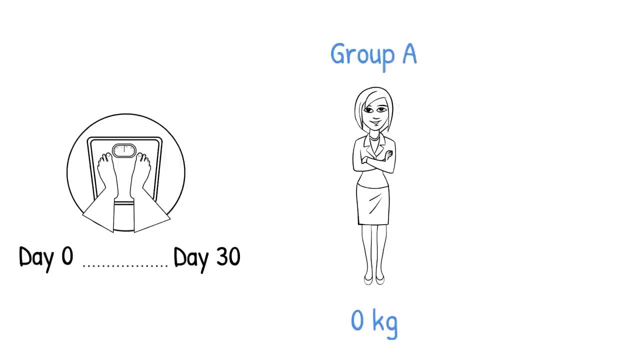 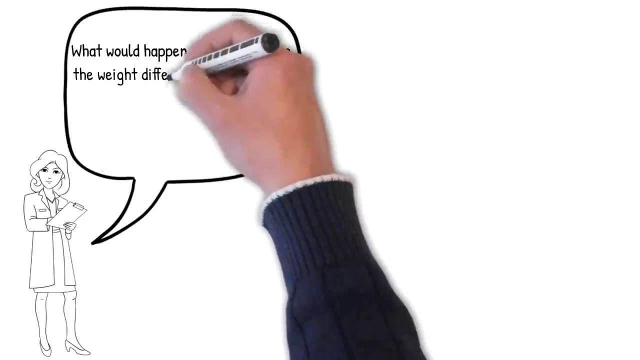 In other words, they did not gain or lose any body weight. Group B's body weight difference was negative one kilogram, So on average they lost one kilogram of their body weight. So does this mean that the drug worked? To determine this, we first ask ourselves what would happen in a world where the weight 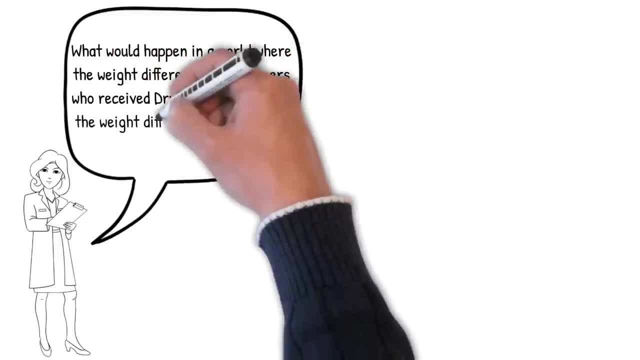 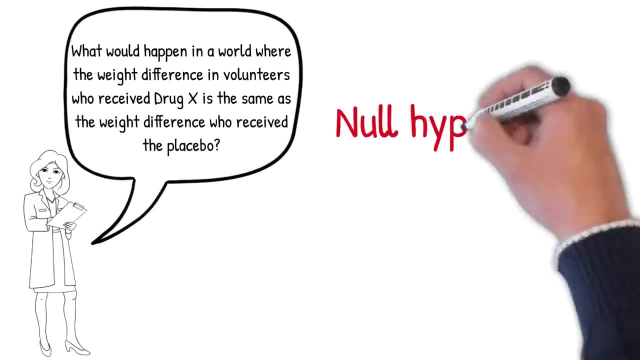 difference in volunteers who received drug X is the same as the weight difference in volunteers who received the placebo. This is where the null hypothesis comes in. Usually, the null hypothesis states that there are no difference between groups, for example. So our null hypothesis is that the weight difference in those who receive 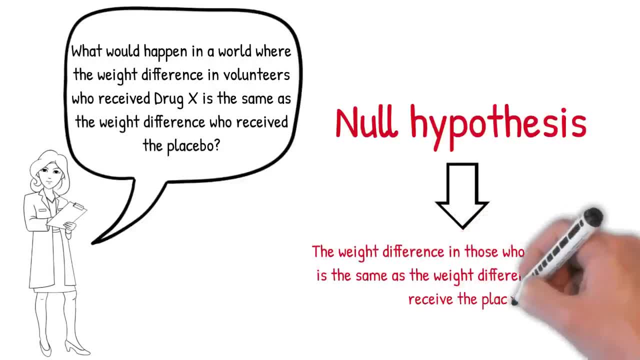 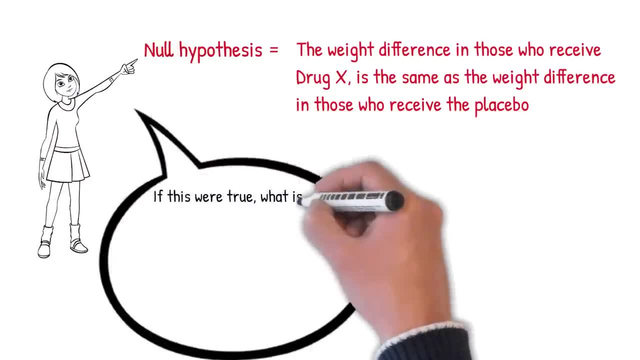 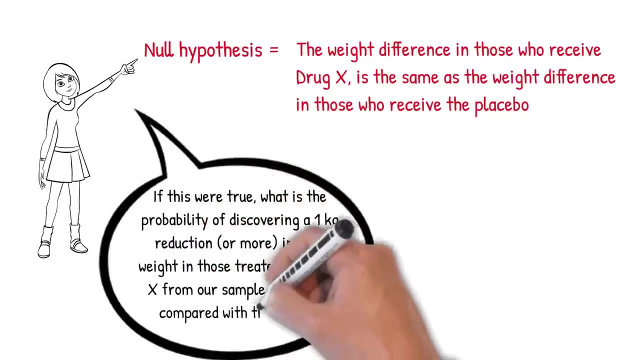 drug X is the same as the weight difference in those who receive the placebo. Now we can ask ourselves: if this null hypothesis were true, what is the chance or probability of discovering a one kilogram reduction or more in body weight in those treated with drug X from our sample? 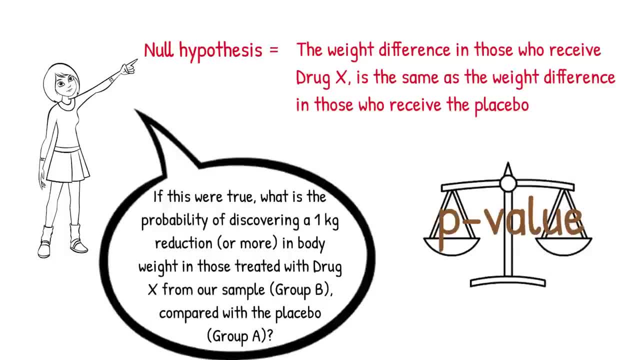 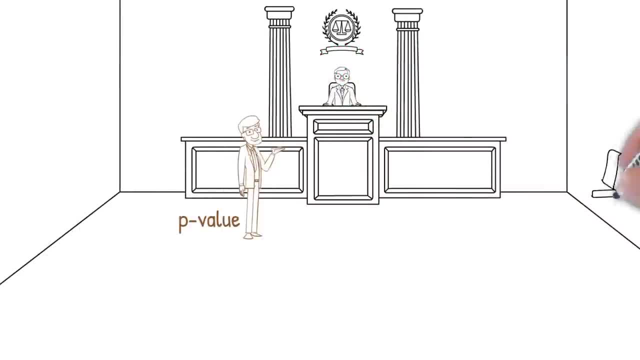 This probability or p-value measures the strength of evidence against the null hypothesis, And you can think of this as a court trial where the defendant is innocent until proven guilty. In this case, the defendant is the null hypothesis. The smaller the p-value, the stronger the evidence against the null hypothesis. 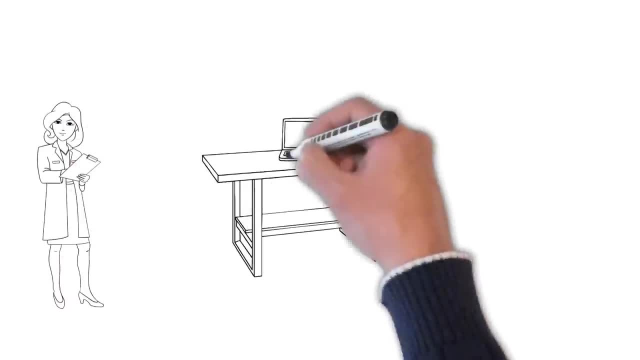 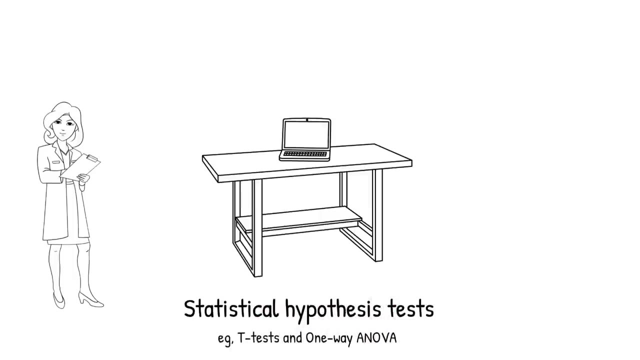 To determine the p-value, scientists use what are known as statistical hypothesis tests. Common examples include the student t-test and a one-way in over. Since this is a top line overview, I will not bombard you with statistical jargon, but instead pretend we have performed a statistical test using our data. 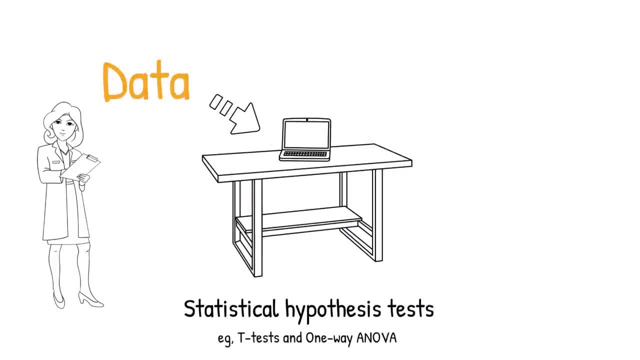 So, after inputting our data into a statistical test, we get a p-value in return. Let's say, for example, the p-value is 0.02.. It's worth mentioning that the p-value is a fraction. However, it may be easier to convert. 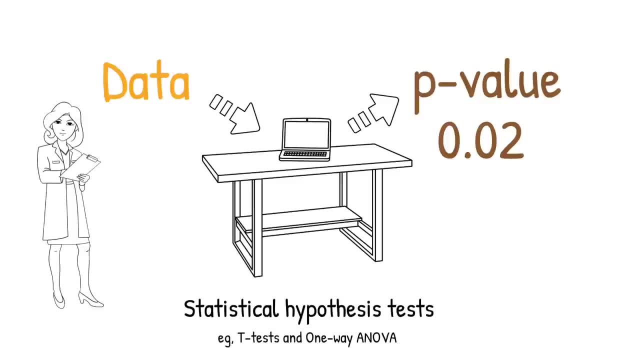 this to a percentage, to simply understand the concept better. So a value of 0.02 would be 2%. I simply multiplied the fraction by 100.. But what does this p-value result of 0.02, or 2% actually represent? 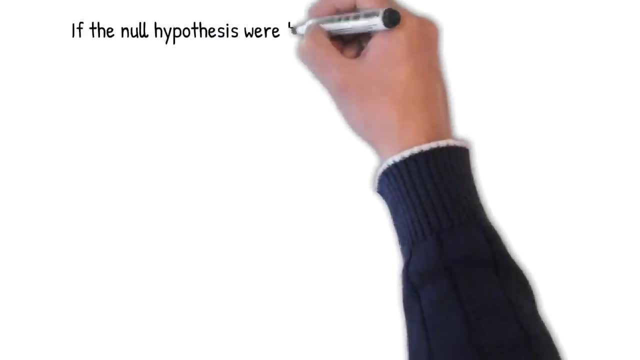 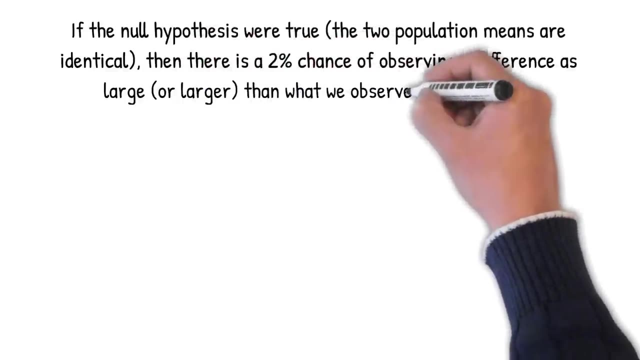 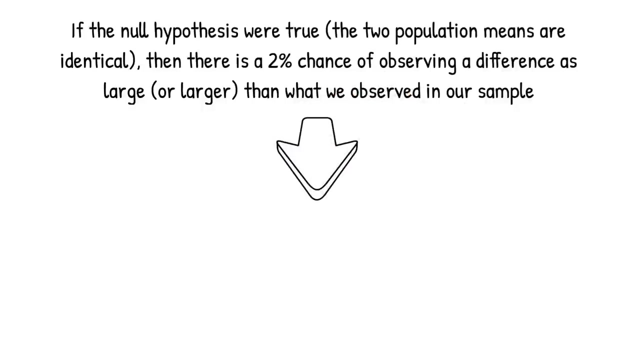 Essentially, this means that if the null hypothesis were true, in other words, that the two population means are identical, then there is a 2% chance of observing a difference as large or larger than what we observed in our sample. In our example, this would translate to: 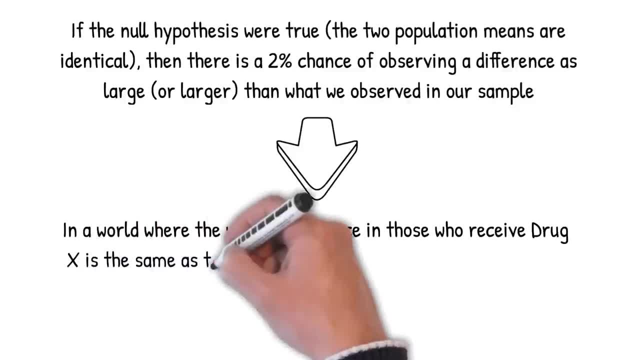 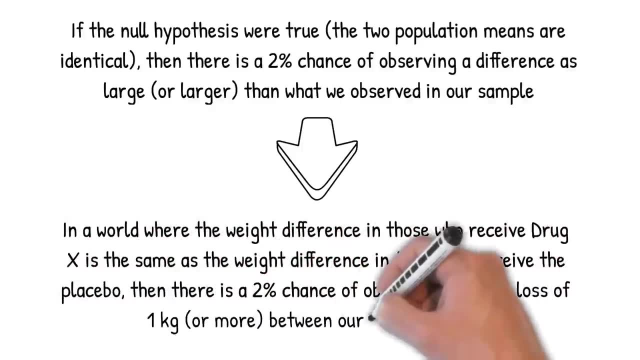 In a world where the weight difference in those who receive drug X is the same as the weight difference in those who receive the placebo, then there is a 2% chance of observing a weight loss of 1 kilogram or more between our sample groups. To put that into perspective, a 2% chance is 1 in every 50 experiments.